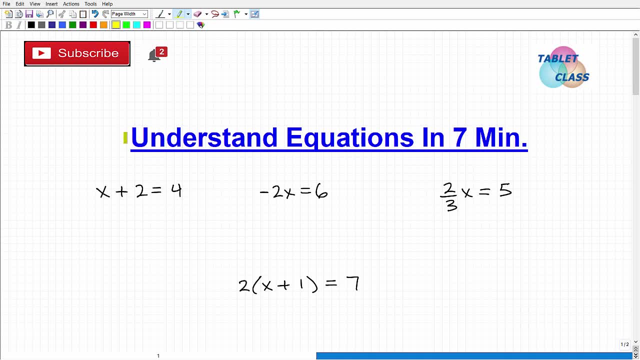 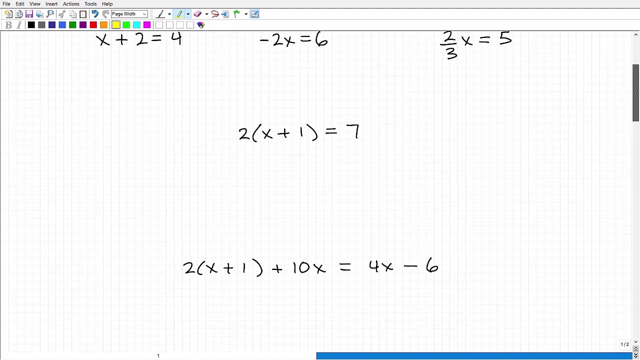 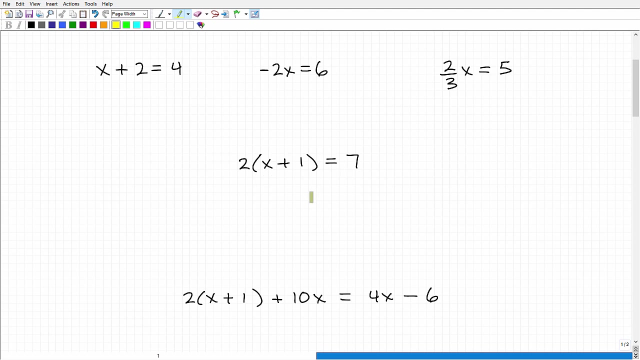 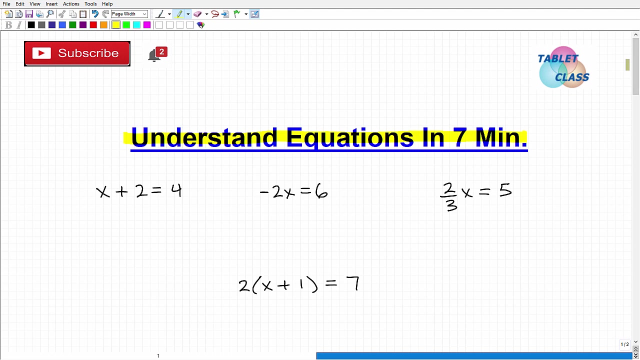 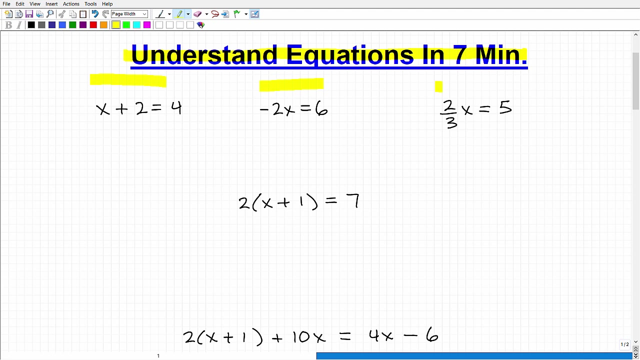 Okay, let's go ahead and see if we can understand basic equations in seven minutes. Now the topic of equations in mathematics is huge, so there's no way I could teach you all different types of equations like quadratic equations, logarithmic equations. It's impossible, but we certainly can kind of review and emphasize some of the things that you need to understand with more basic algebraic type of equations in a short period of time. So my goal here is to do these questions in seven minutes. Okay, so we'll start out with some real basic ones, make sure you understand the fundamentals, and then we'll go on to a little bit more interesting problems. But with this, I'll be able to emphasize some things that I see students really struggle with because they don't understand the basics. That's why they have problems with more challenging problems. So let's go ahead and just really make sure you strengthen your fundamentals in equations. Okay, so let's go ahead and just really make sure you strengthen your fundamentals in equations. Now let me state one thing here. This is probably for somebody that's at the pre-algebra, algebra one level, or maybe another course. But I teach equations really thoroughly in my algebra course, not just these type of equations, but other types, quadratic equations, etc. So I'm going to leave a link to that course in a description of this video. But before we get going, let me introduce myself. My name is John. I'm the founder of Tablet Class Math. My name is John. I'm the founder of Tablet Class Math. I'm also a middle and high school math teacher. So I've been teaching this stuff for many, many, many years. So let's get into it now. All right, so here I have three basic type of equations. I would suggest if you want to maybe pause the video and see if you can do these three equations. Okay, just check your current level of understanding. Okay, make sure you show your work. But let me go ahead and get into it now. All right, so here I have x plus two equals four. When I'm 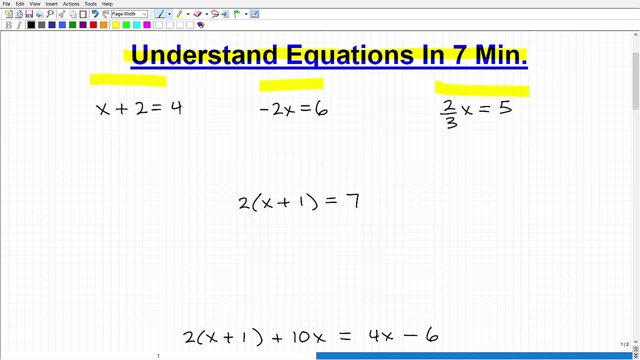 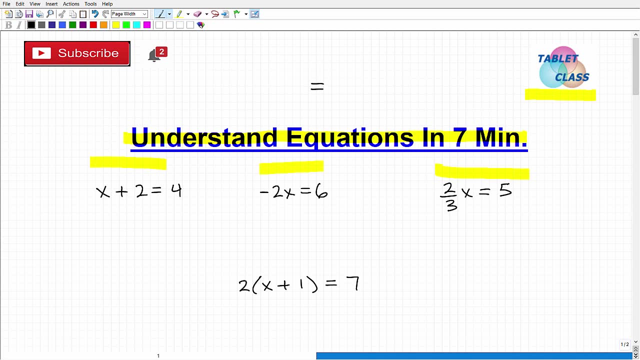 talking about equations, I'm talking about solving equations. All right, Now let me just state something here real quick. All right, in an equation here we have a variable we're trying to. the goal is to try to find the value of x. okay, the value of x is going to be some number And that number, if it is in fact the solution, is going to make the equation true. In other words, when we plug in that number, replace all any x value in the equation. when we plug it in, it's true. 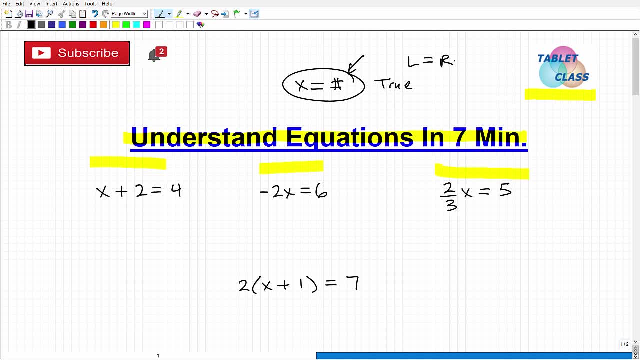 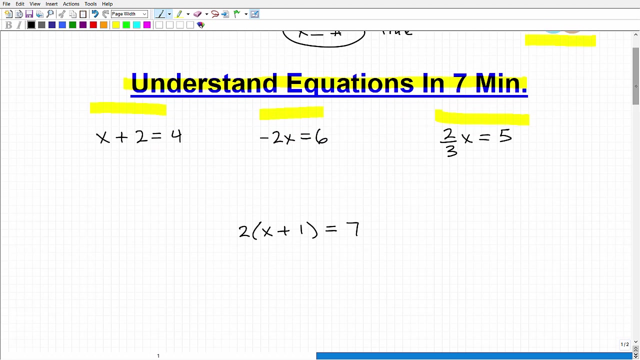 If the left hand side equals the right hand side. So that's the main concept of trying to solve an equation. Another thing about equations is this: In algebra, whatever you do to one side of the equation- okay, for example, the left hand side- you have to do the exact same thing to the right hand side. So these are real fundamental concepts, But again, you know this is a short video, So so much more to cover, But let's get into the mechanics right now. All right, first thing is 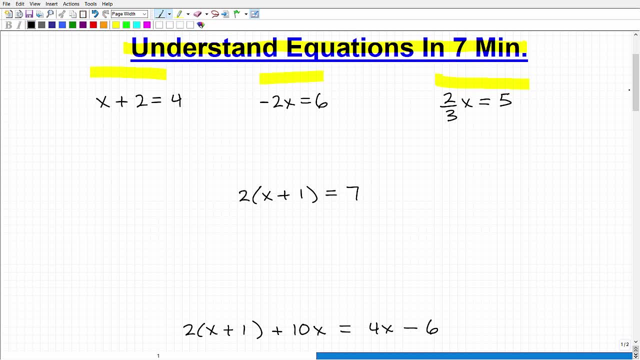 when you're solving equations, make sure you show all your work. That's really critical and be super neat. So here we go. we got x plus two equals four. The way I want to solve that is: I'm going to subtract two from both sides of the equation And I get x is equal to two. Okay, you want to show your work, just like this. Remember, the objective is I want to get x equal to some value, And what I did here was I subtracted two from both sides of the equation. 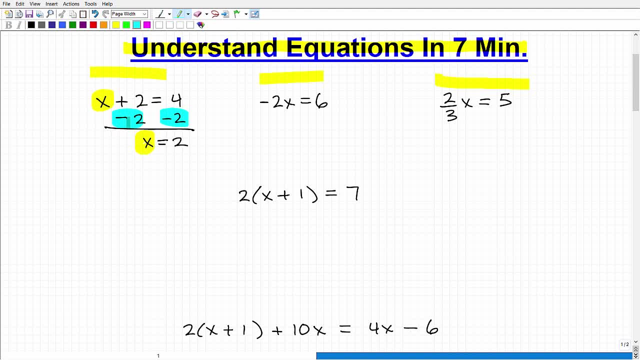 Remember, whatever you do on one side of the equation, you have to do to the other side of the equation as well. Now I'm skipping over a lot of other critical things here, But you know, again, I'm assuming you already have some knowledge of equations right now. Okay, so the objective here really is to focus on the process or the mechanics, not so much the theory. Okay, I'm kind of trying to hit that a little bit, But let's continue on with our second problem. Okay, so how do we solve this negative two x? 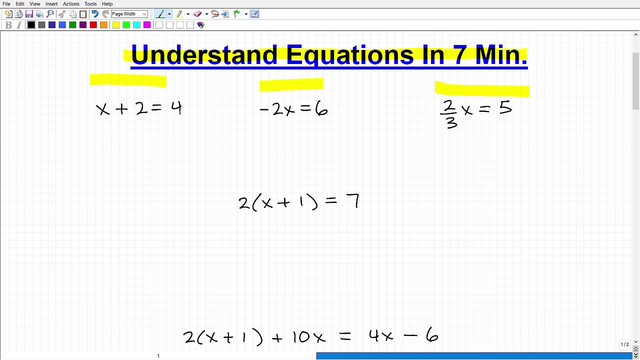 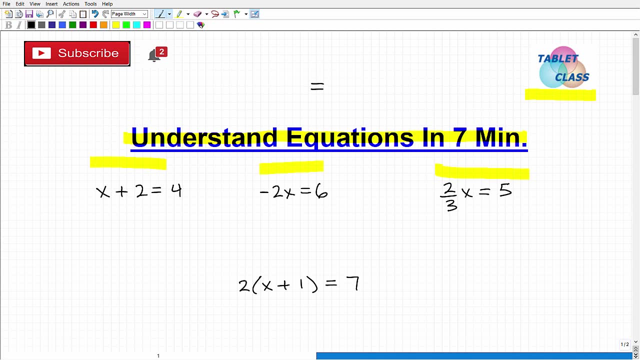 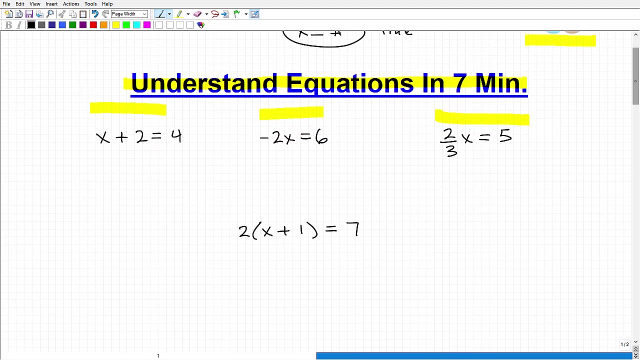 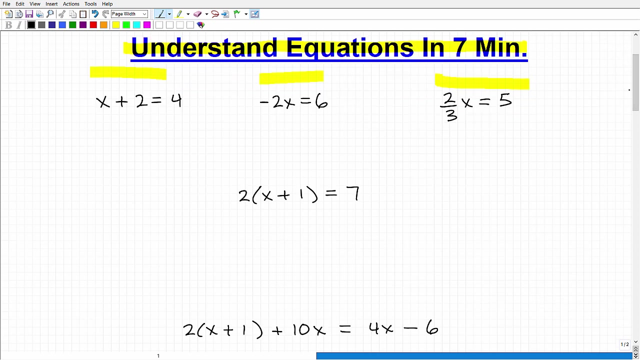 talking about equations, I'm talking about solving equations. All right. Now let me just state something here real quick. All right, in an equation, here we have a variable, we're trying to the goal is to try to find the value of x, okay, the value of x is going to be some number. And that number, if it is, in fact, the solution is going to make the equation true. In other words, when we plug in that number, replace all any x value in the equation, when we plug it in, it's true. If the left hand side equals the right hand side. So that's the main concept of trying to solve an equation. Another thing about equations is this. In algebra, whatever you do to one side of the equation, okay, for example, the left hand side, you have to do the exact same thing to the right hand side. So these are real fundamental concepts. But again, you know, this is a short video. So, so much more to cover. But let's get into the mechanics right now. All right, first thing is, when you're solving equations, make sure you show all your work. That's really critical, and be super neat. So here we go, we got x plus two equals four. The way I want to solve that is I'm going to subtract two from both sides of the equation. And I get x is equal to two. Okay, you want to show your work just like this. Remember, the objective is, I want to get x equal to some value. And what I did here was I subtracted two from both sides of the equation. 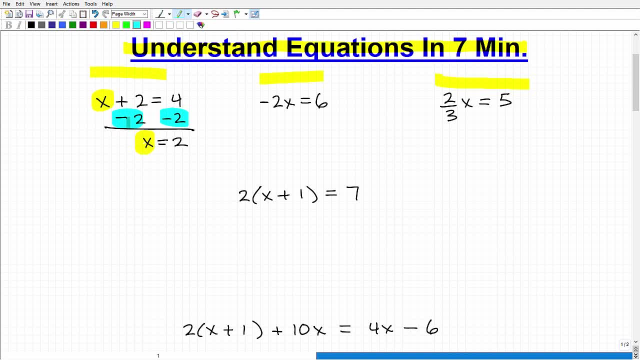 Remember, whatever you do on one side of the equation, you have to do to the other side of the equation as well. Now I'm skipping over a lot of other critical things here. But you know, again, I'm assuming you already have some knowledge of equations right now. Okay, so the objective here really is to focus on the process or the mechanics, not so much the theory. Okay, I'm kind of trying to hit that a little bit. But let's continue on with our second problem. Okay, so how do we solve this negative two x, equals six? Well, in this equation, I need to divide both sides of the equation by negative two. Okay. Now, one thing I want to say is that you really make sure you know your positive and negative numbers really, really well. Because that's another place where students kind of trip up with the equation. So negative two divided by negative two is positive one, or positive one x, that's going to be x is equal to negative three. Okay, so that's the solution to this equation. Now, let's move on to this last one. Now, here, okay, what I had to do was do some subtraction to both sides of the equation. Here, I had to do some division. Okay, I'm dividing. Now in this equation right here, the best way to solve an equation where there's a fraction in front of the variable like so, is just to flip that fraction, we call that the reciprocal. So that's going to be three over two. And we're going to multiply both sides of the equation by the reciprocal. So whatever this number is here, flip it upside down, or either reciprocal. And then you want to multiply both sides of the equation by the reciprocal. So we're going to take this five and multiply it by three halves. Five is the same thing as five over one. So here, three halves times two thirds is one or one, one x or just x. And this is going to be 15 over two or 15 halves. Okay, so that is the 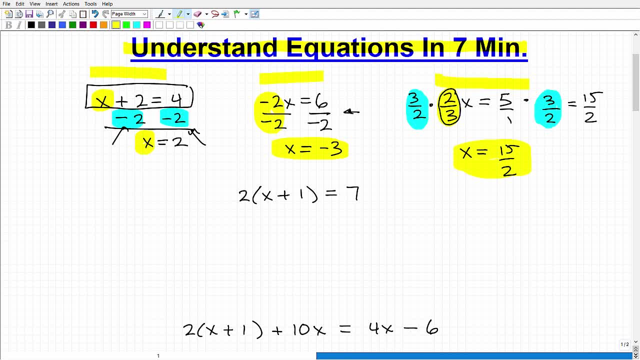 solution to this equation here. So make sure you understand the basics because with equations, 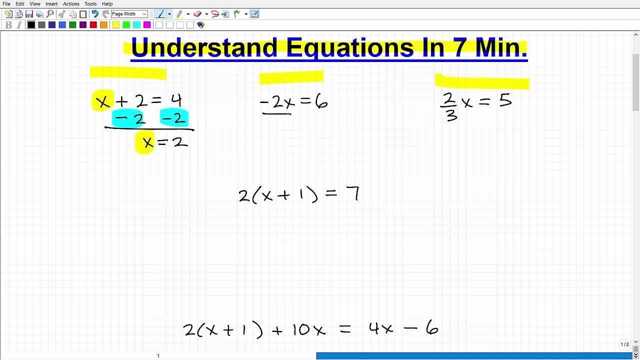 equals six. Well, in this equation I need to divide both sides of the equation by negative two. Okay. Now one thing I want to say is that you really make sure you know your positive and negative numbers really really well, Because that's another place where students kind of trip up with the equation. So negative two divided by negative two is positive one or positive one, x that's going to be. x is equal to negative three. Okay, so that's the solution to this equation. Now let's 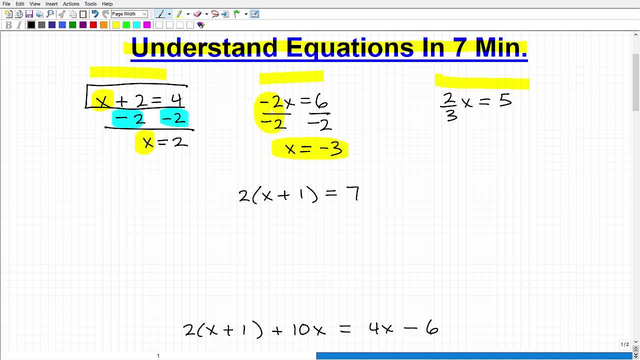 move on to this last one Now here. okay, what I had to do was do some subtraction to both sides of the equation. Here I had to do some division. Okay, I'm dividing Now in this equation right here. the best way to solve an equation where there's a fraction in front of the variable, like so, is just to flip that fraction. we call that the reciprocal. So that's going to be three over two And we're going to multiply both sides of the equation by the reciprocal, So whatever. 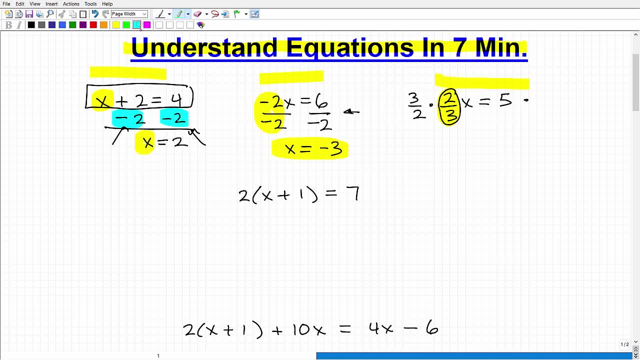 this number is here, flip it upside down or either reciprocal, And then you want to multiply both sides of the equation by the reciprocal. So we're going to take this five and multiply it by three halves. Five is the same thing as five over one. So here, three halves times two thirds is one. 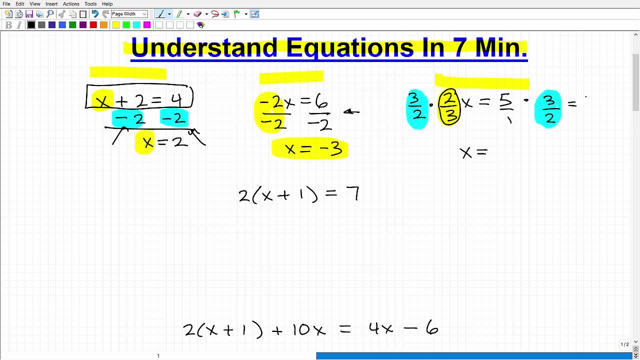 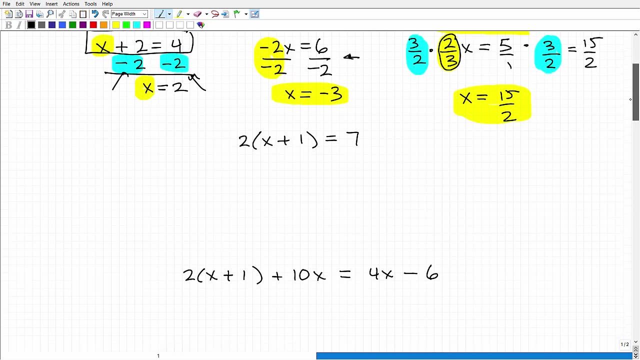 or one, one x or just x, And this is going to be 15 over two or 15 halves. Okay, so that is the solution to this equation here. So make sure you understand the basics, because with equations, linear equations, we're just taking a. let's say something like what I'm going to do down here. 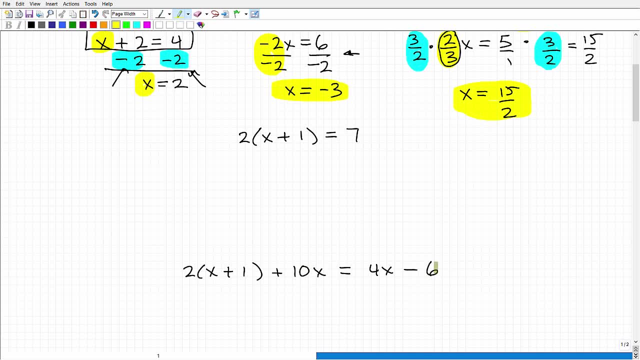 you're taking a big equation and just chipping away at it, rewriting it one step at a time until it becomes a small equation, But the steps that we're doing are generally the same. Okay, we're just kind of having to manage the problem down, Alright. so what about an equation like this? 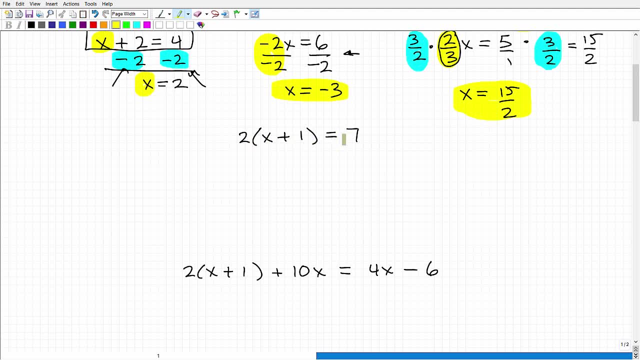 right, x plus one equals seven. Well, in algebra, anytime you see parentheses like so, this is an indication that you have to do the distributor property before you do anything else. So let's go ahead and do that now. So this is going to be two times x, or two x plus two times one. Alright, so that's. 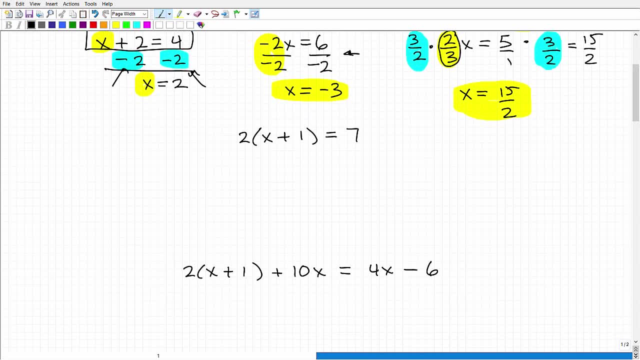 linear equations, we're just taking a, let's say something like what I'm going to do down here, you're taking a big equation and just chipping away at it, rewriting it one step at a time until it becomes a small equation. But the steps that we're doing are generally the same. Okay, we're just kind of having to manage the problem down. Alright, so what about an equation like this, right? 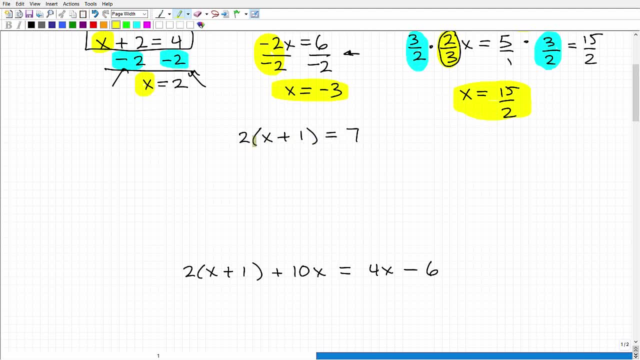 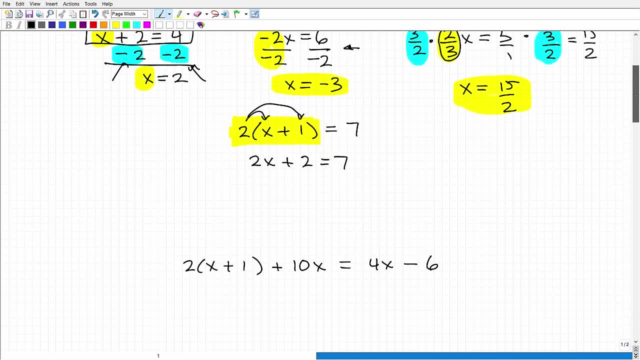 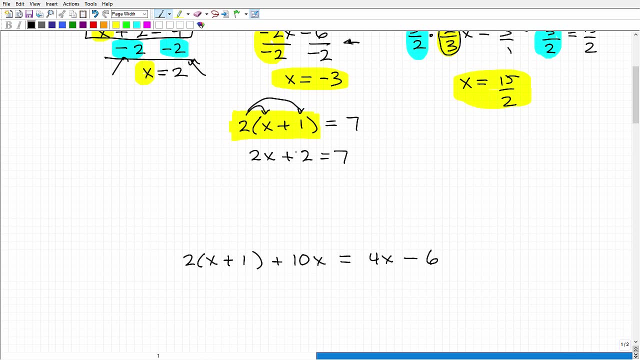 And apply the distributor property when necessary. But at this point, I'm like, okay, what do I do now? Well, here, we always take care of addition or subtraction first. So I'm going to get rid of this two by subtracting two from both sides of the equation. And that's going to give me, let me scoot this guy down here a little bit. This is going to give me two x is equal to five. Alright, 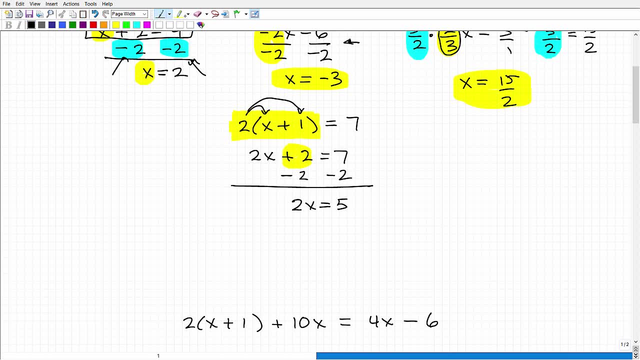 see how I'm kind of writing this down. And now here, this is a basic equation, something that we did like up here, or we just take another step. 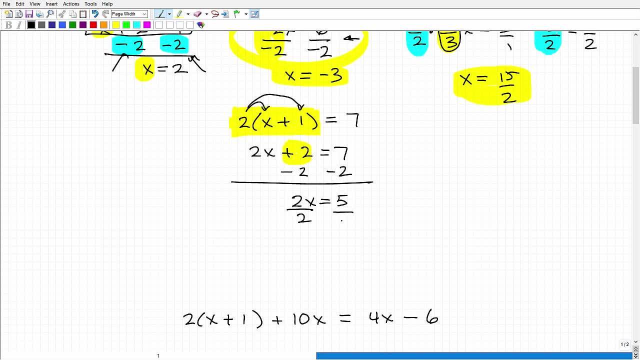 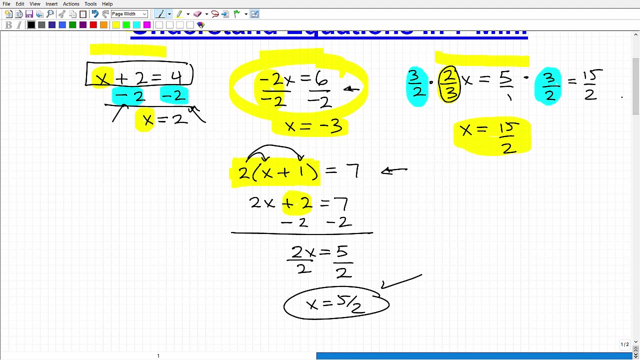 And to solve for x, I just simply divide both sides of the equation by two. So I get x is equal to five halves. And there you go. Okay, so, again, just another kind of step up in how many steps we have to take to solve an equation. So let's go ahead and finish this video up with this equation here. 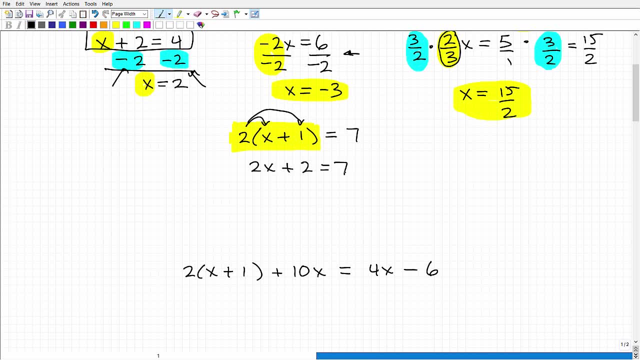 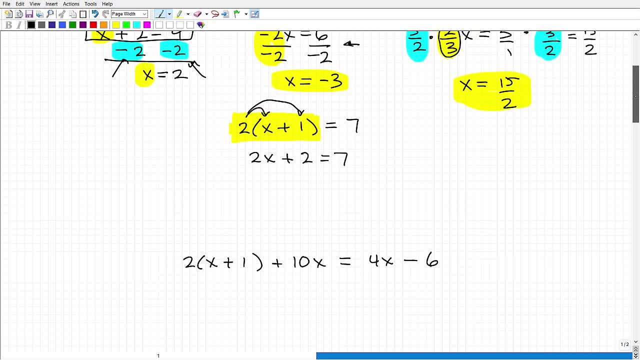 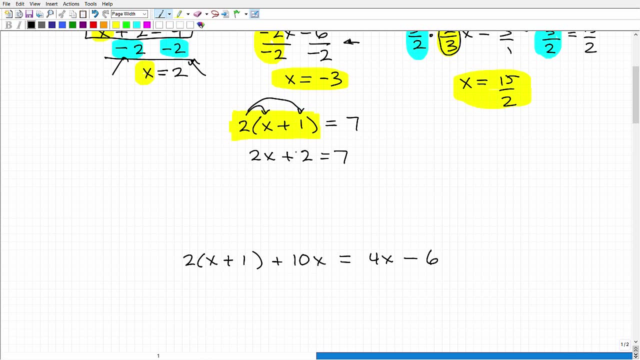 And apply the distributor property when necessary. But at this point I'm like, okay, what do I do now? Well here, we always take care of addition or subtraction first. So I'm going to get rid of this two by subtracting two from both sides of the equation, And that's going to give me- let me. 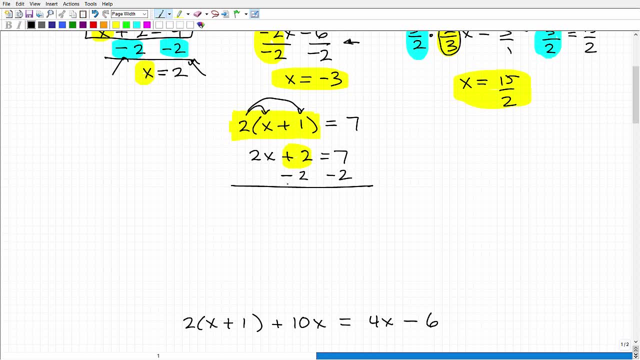 scoot this guy down here a little bit. This is going to give me two. x is equal to five. Alright, see how I'm kind of writing this down. And now here, this is a basic equation, something that we did like up here, or we just take another step. 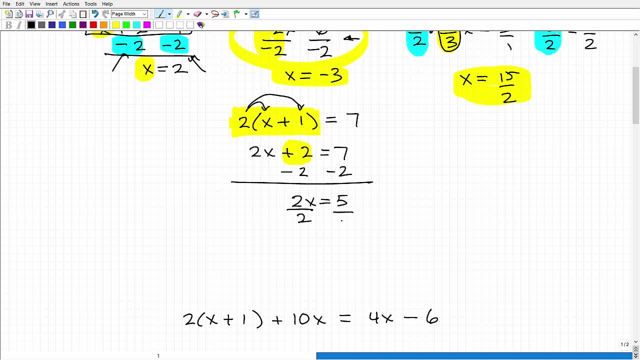 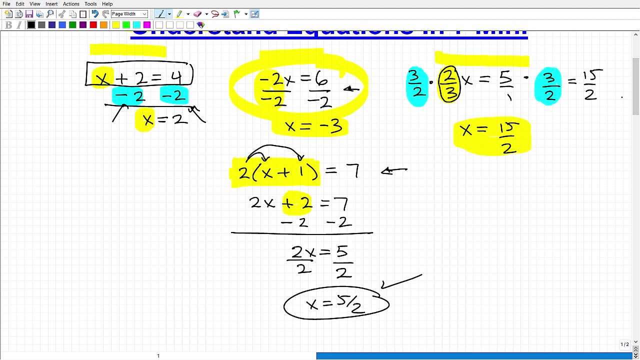 And to solve for x, I just simply divide both sides of the equation by two, So I get x is equal to five halves. And there you go. Okay, so again just another kind of step up in how many steps we have to take to solve an equation. So let's go ahead and finish this video up with this equation. 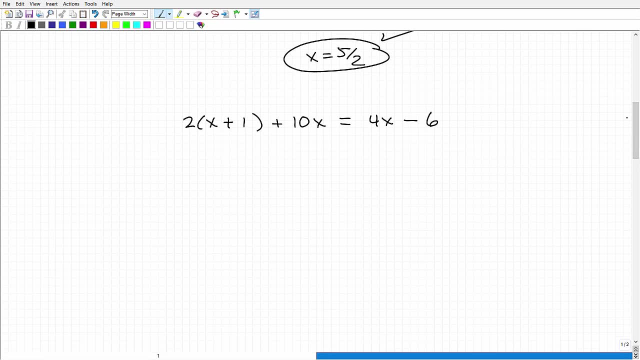 here, Because again there's all kinds of different twists and things, But again you're using the same fundamental steps over and over again to kind of whittle the problem down, if you will. Alright. so here I have an equation And, as I said previously, if I see parentheses like so, 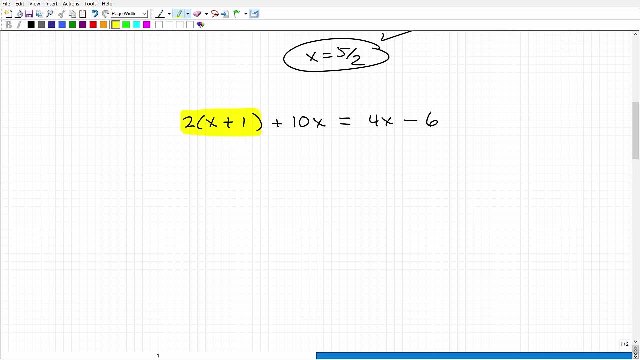 quantity. this is an indication. I'm going to have to do the distributor property first, So let's start off this way. So I'm going to have to multiply that two by x and one, So it's going to be two times x, or two x plus two. 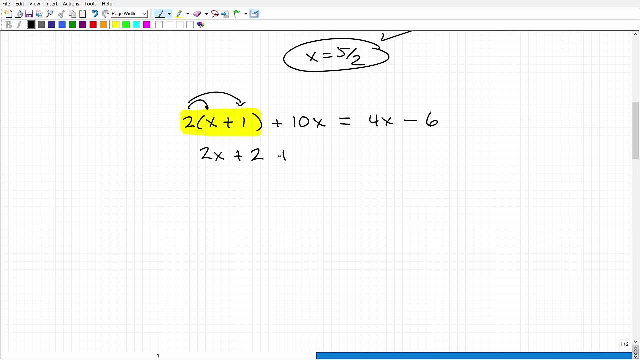 times 1,, that's 2.. Now let's just write the rest of the equation out: Plus 10x is equal to 4x minus 6.. Okay, now, at this time, what you want to do is you want to combine like terms. So we have. 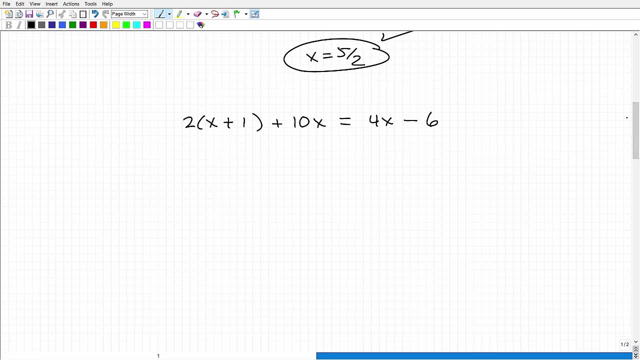 Okay, so what I want to do is, again, there's all kinds of different twists and things. But again, you're using the same fundamental steps over and over again, to kind of whittle the problem down, if you will. Alright, so here I have an equation. And as I said previously, if I see parentheses like so quantity, this is an indication, I'm going to have to do the distributor property first. So let's start off this way. So I'm going to have to multiply by that two by x and one, so it's gonna be two times x or two x, plus two, times 1, that's 2. Now let's just write the rest of the equation out. Plus 10x is equal to 4x minus 6. Okay, now at this time, what you want to do is you want to combine like terms. So we have the left and right hand side of the equation. We want to simplify each of those sides by adding anything that we can on the respective sides before we do anything else. So in this case, 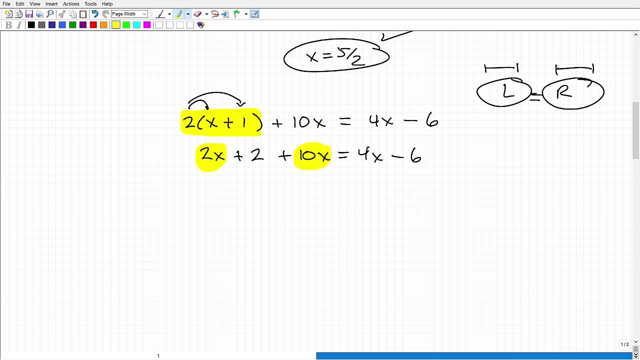 I have this 2x and I have this 10x. So these are like terms. I can add these together. A 2x and a 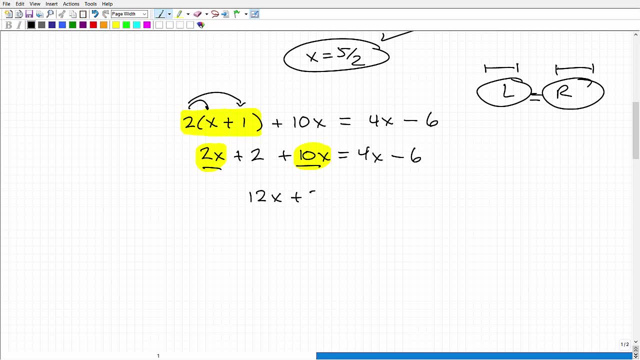 10x is 12x plus 2 is equal to 4x minus 6. So here I have a 4x and a minus 6. I can't combine these 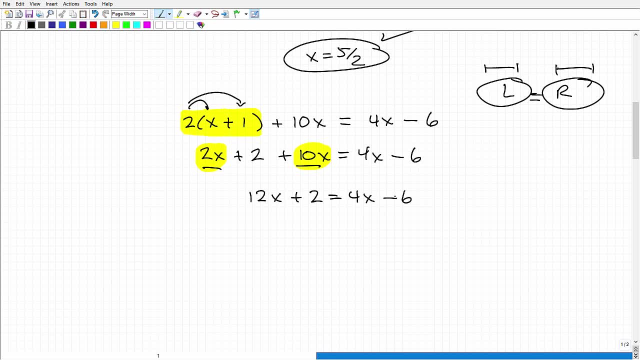 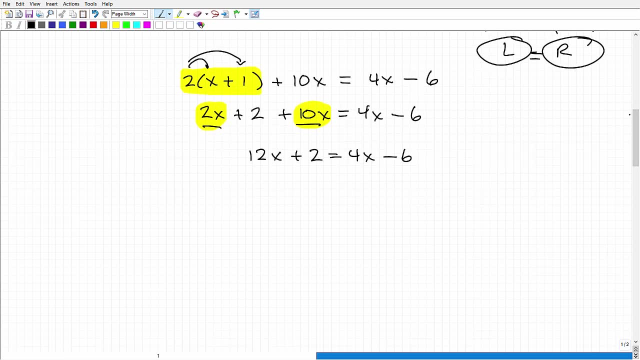 because these are not like terms. Again, I'm kind of skipping over a lot of things, but I'm kind of making that assumption that you have some sort of idea already of what's going on with equations, right? We're just kind of doing a quick, 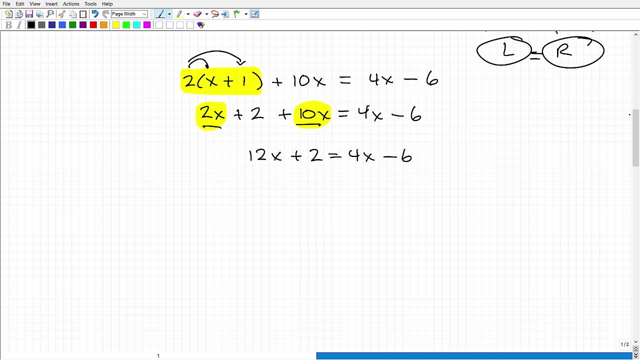 review here with this video. All right, now at this point, what you want to do is you want to move all your variables, okay, over to the left hand side and move all the numbers over to the right hand side. So let's go ahead and start with the variables first. So I have this 4x on the right hand side. I want to move it over to the left hand side. So the way I'm going to do that, I'm going to subtract the 4x over here. But if I do a subtraction on the right hand side, I'm going to have to do it over here. 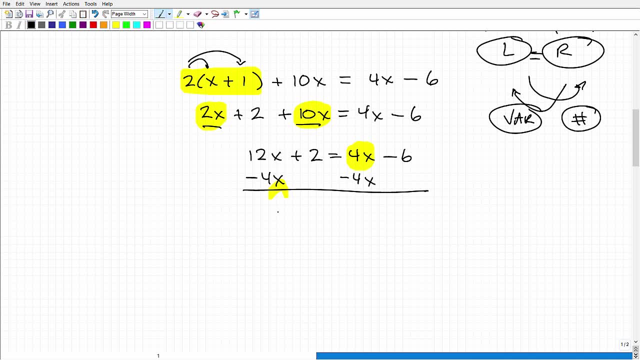 So this is going to be 8x plus 2 is equal to negative 6. So I just move my 4x over to the left hand side. And now I just want to move all my numbers over to the right hand side. 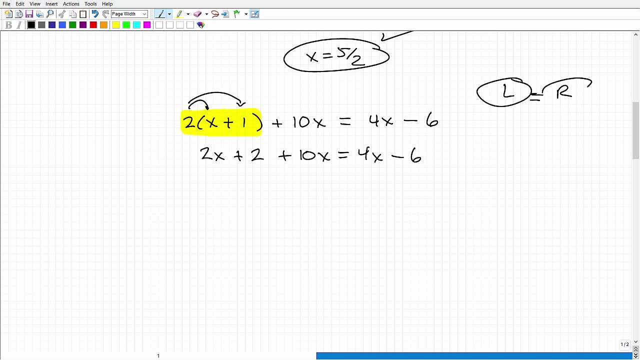 the left and right hand side of the equation. We want to simplify each of those sides by adding anything that we can on the respective sides before we do anything else. So in this case, I have this 2x and I have this 10x. So these are like terms. I can add these together: A, 2x and a. 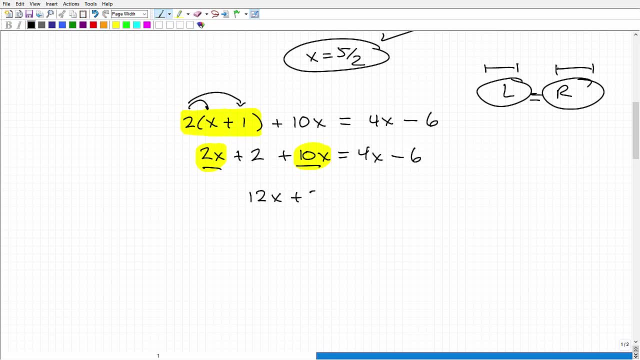 10x is 12x plus 2 is equal to 4x minus 6.. So here I have a 4x and a minus 6. I can't combine these because these are not like terms. Again, I'm kind of skipping over a lot of things, but I'm kind of. 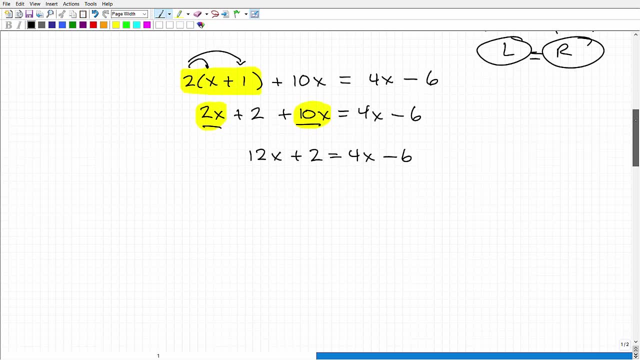 making that assumption that you have some sort of idea already of what's going on with equations. right, We're just kind of doing a quick review here with this video. All right now, at this point, what you want to do is you want to. 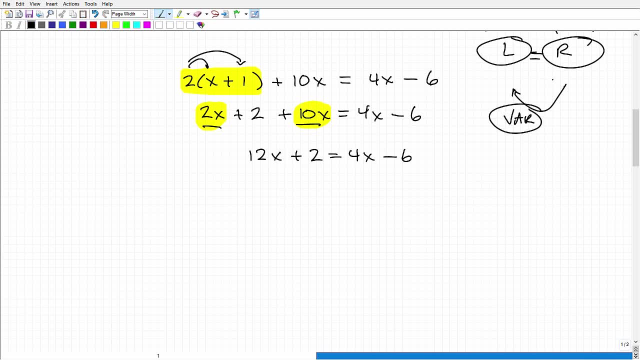 move all your variables, okay, over to the left hand side and move all the numbers over to the right hand side. So let's go ahead and start with the variables first. So I have this 4x on the right hand side, I want to move it over to the left hand side. So the way I'm going to do that, 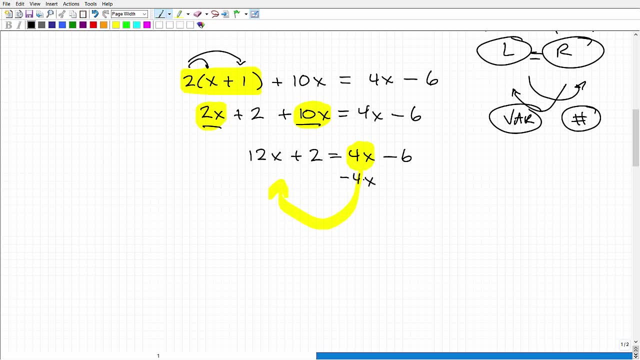 I'm going to subtract the 4x over here. But if I do a subtraction on the right hand side, I'm going to have to do it over here. So this is going to be: 8x plus 2 is equal to negative 6.. So I just move my 4x over to the 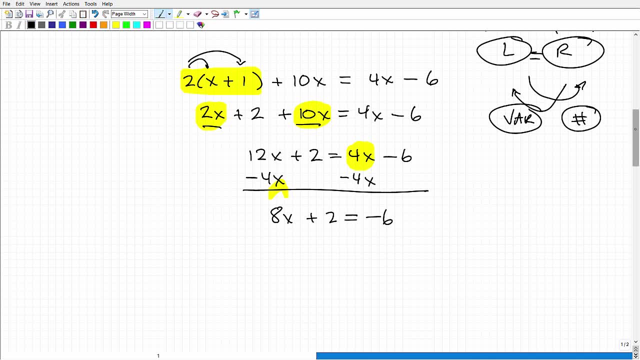 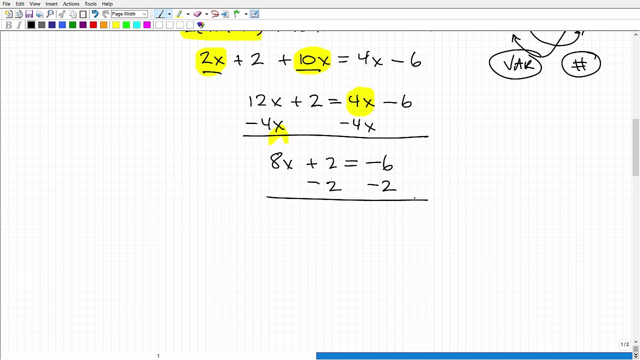 left hand side, And now I just want to move all my numbers over to the right hand side. So I'm going to subtract 2 from both sides of the equation like so, And I'm going to get: 8x is equal to negative 8.. All right, And last but not least, 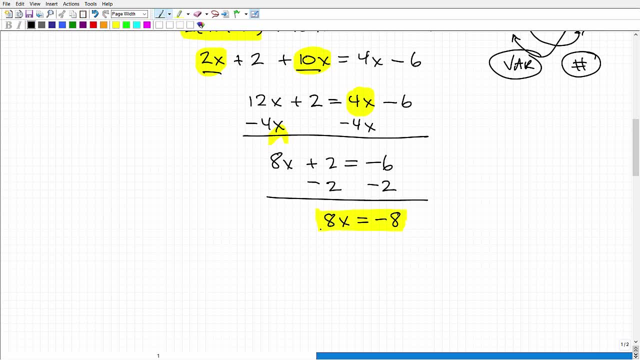 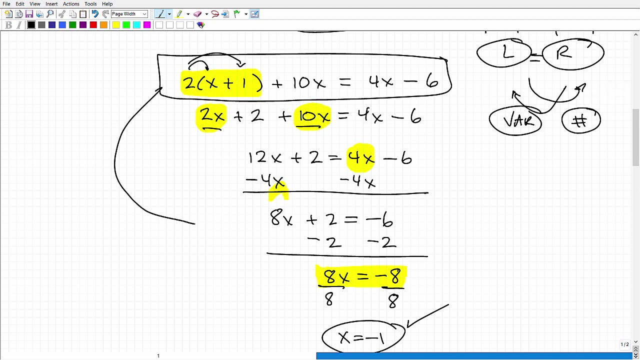 now I have this real basic equation. I'm going to go ahead and divide both sides of the equation by 8. And I get: x is equal to negative 1. That is the solution. So what you're doing is you're taking this big equation and you're just continuing to rewrite it in a more simpler 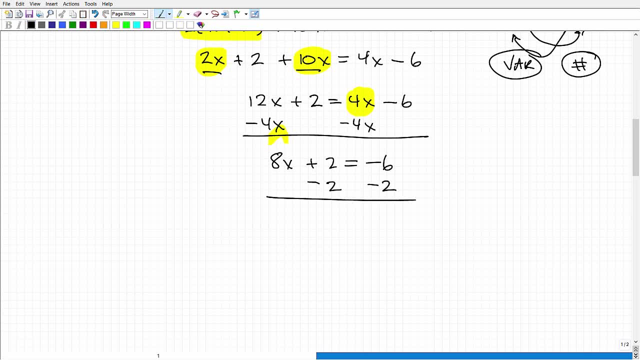 So I'm going to subtract 2 from both sides of the equation like so. And I'm going to get 8x is equal 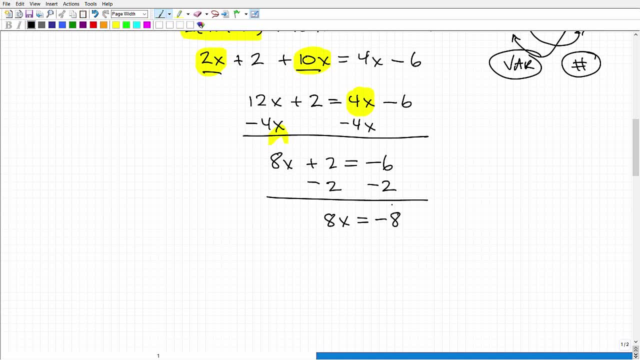 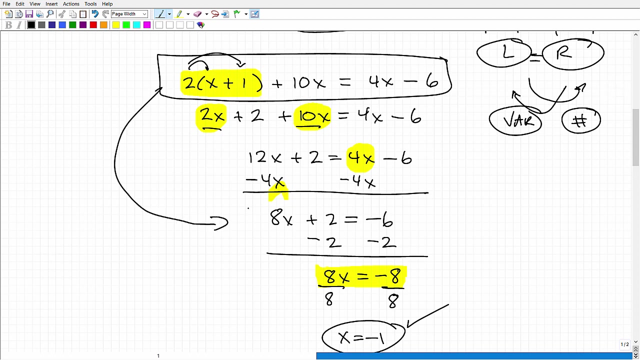 to negative 8. All right. And last but not least, now I have this real basic equation. I'm going to go ahead and divide both sides of the equation by 8. And I get x is equal to negative 1. That is the solution. So what you're doing is you're taking this big equation, and you're just continuing to rewrite it in a more simpler and simpler manner until you can actually solve the equation. All right, until you actually get 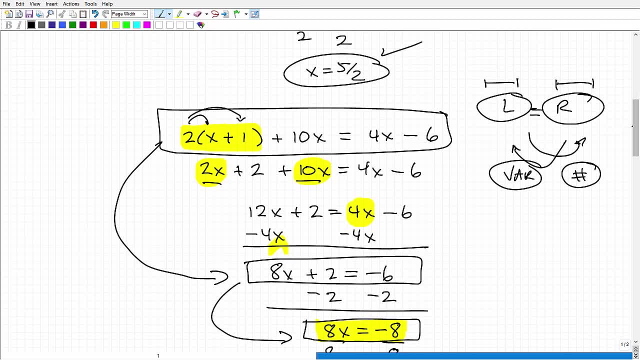 to the solution. So it's not, you know, when you're doing this, you're not going to get to the solution. 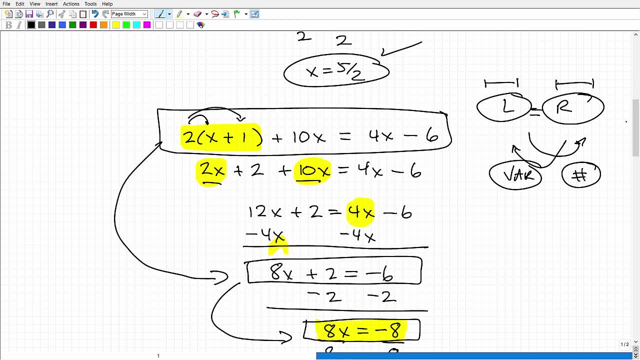 Of course, you could have fractions involved and decimals, etc. But where I see students really struggle is they don't even, you know, really have the fundamentals down. So if you're struggling 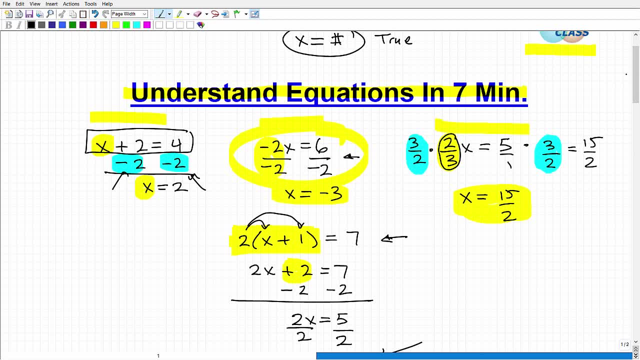 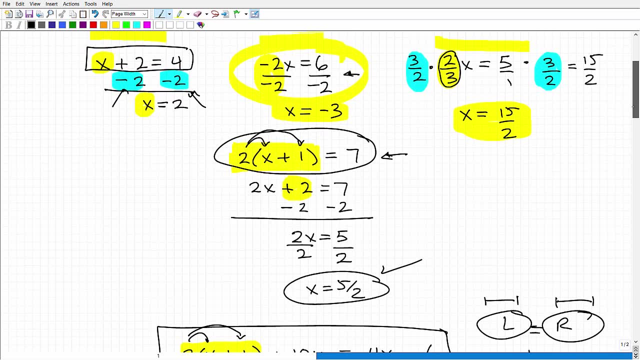 with equations, make sure you get the basics down really, really well. And then, you know, these little more two-step kind of equations, and then you kind of get into the multi-step. 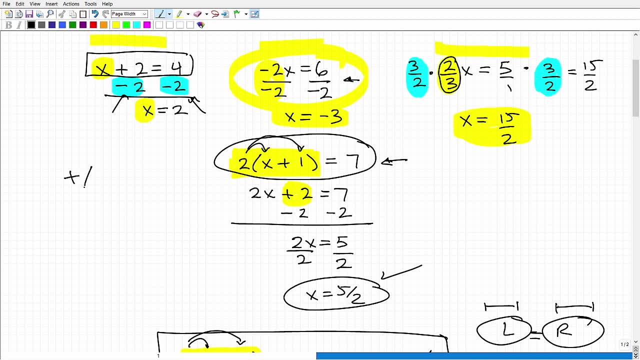 A couple of key areas that students make mistakes is dealing with positive and negative numbers. They do, a lot of students confuse or make errors in solving equations with this. Another place students really make mistakes is the distributive property. Okay, like right here. So make sure you really have that distributive property down. Of 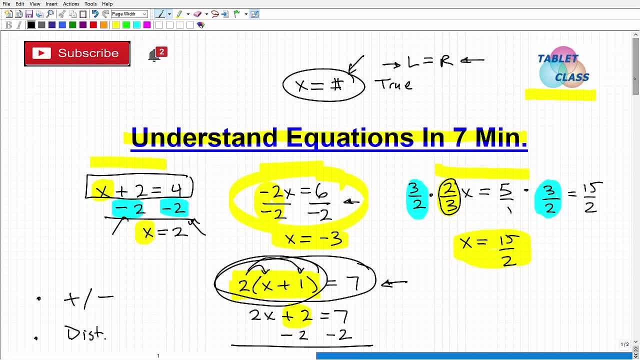 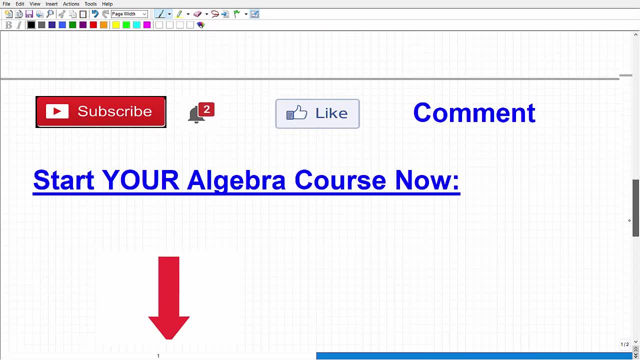 course, I teach all this in my courses. But again, I'm kind of skipping over a lot of things. But hopefully this was a somewhat of a review, useful review for you. But let's go and wrap this video up. At the time of this video, I've been on YouTube for a good 12 years. I've been on YouTube for a good 12 years. 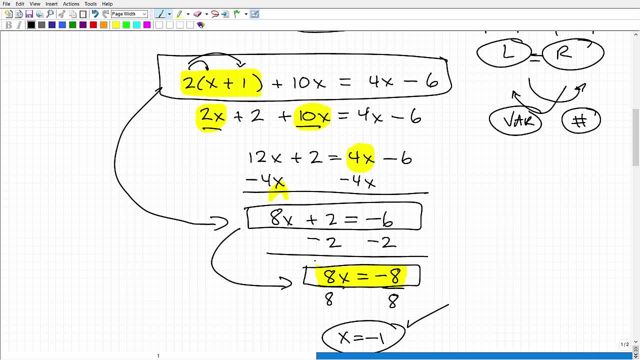 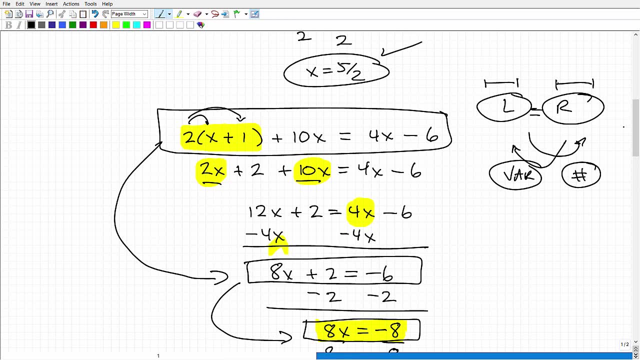 and simpler manner until you can actually solve the equation. All right, until you actually get to the solution. So it's not you know, when you're doing this, you're not going to get to the solution. Of course you could have fractions involved and decimals, etc. But where I see students really 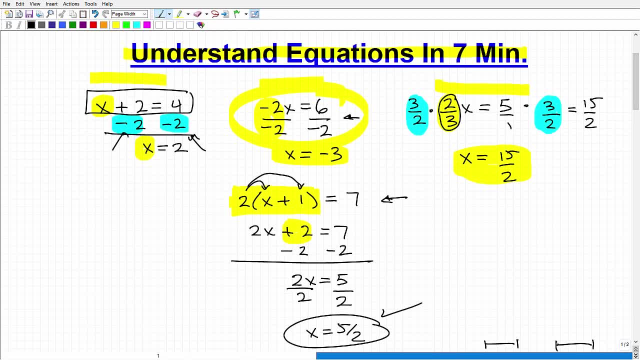 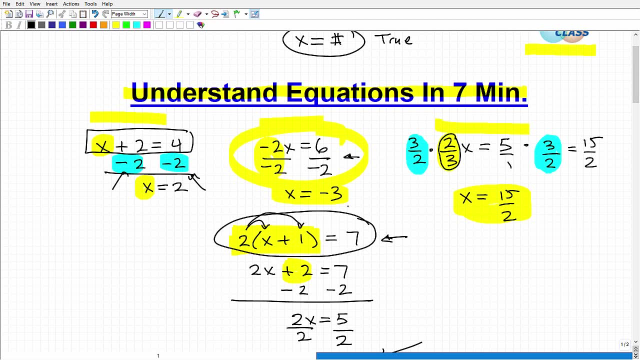 struggle is they don't even, you know, really have the fundamentals down. So if you're struggling with equations, make sure you get the basics down really, really well, And then you know these little more two-step kind of equations and then you kind of get into the multi-step. 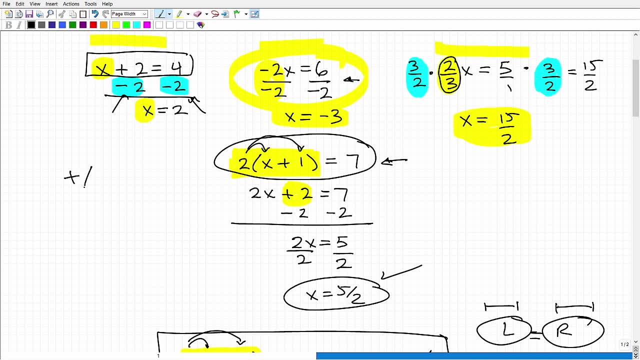 A couple of key areas that students make mistakes is dealing with positive and negative numbers. They do a lot of students confuse or make errors in solving equations with this. Another place students really make mistakes is the distributive property. Okay, like right here. So make sure you really have that distributive property down Of. 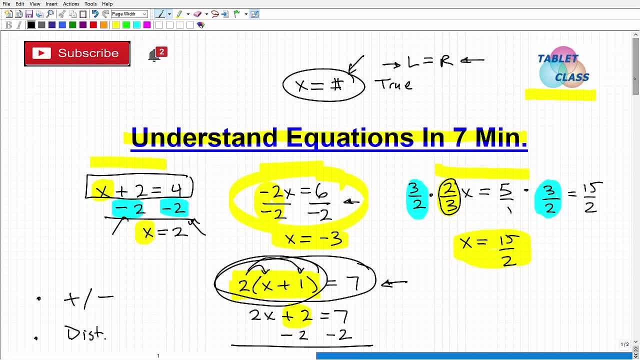 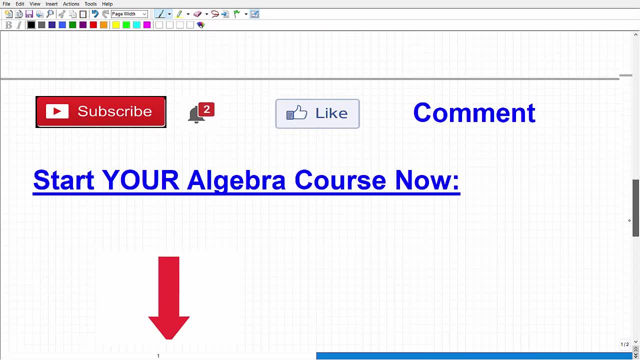 course I teach all this in my courses, But again I'm kind of skipping over a lot of things. But hopefully this was a somewhat of a review, useful review for you. But let's go and wrap this video up. At the time of this video I've been on YouTube for a good 12 years. I've been on YouTube for a. 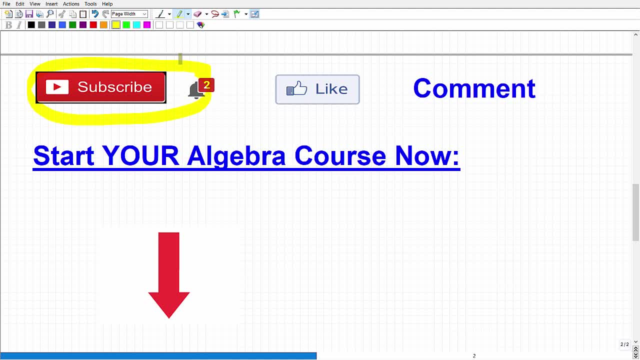 good 12 years, Really love posting my math videos on YouTube And I think I have hundreds and well like six 700 videos on YouTube at this point. But I'm posting content all the time. I really enjoy doing that, So hopefully consider subscribing If you enjoyed this video. 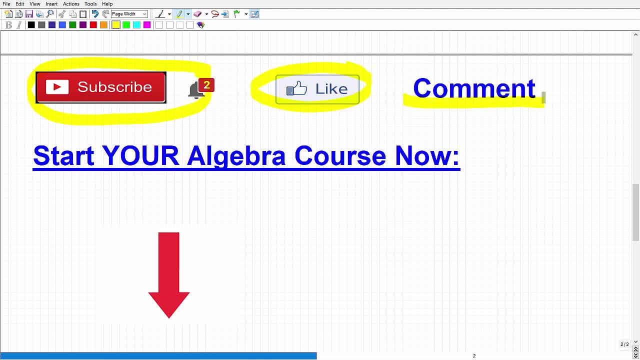 definitely appreciate a thumbs up And leave me some feedback. What course are you in? Are you in pre-algebra, algebra one? Are you going back to school? Maybe you're taking the GED and you're just looking to learn about equations. So I'll see you in the next video. Bye-bye. 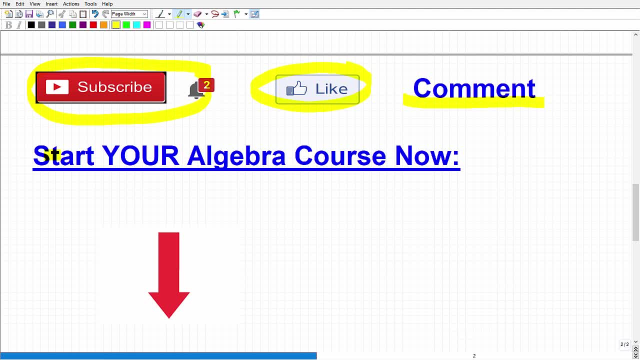 Any feedback is good feedback. And, last but not least, I'm going to leave a link to my algebra course in the description of this video. If you're in pre-algebra, if you just follow that link, it'll take you to my entire course catalog. I literally have over 100 math courses, All my